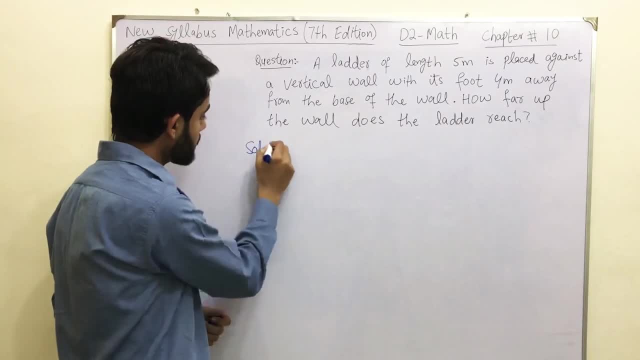 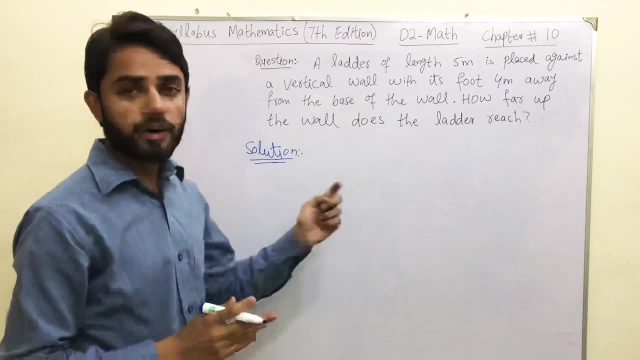 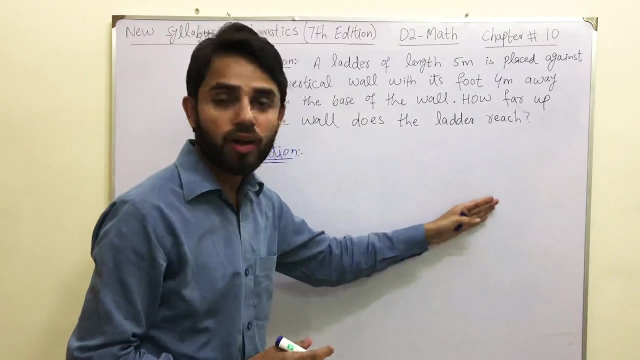 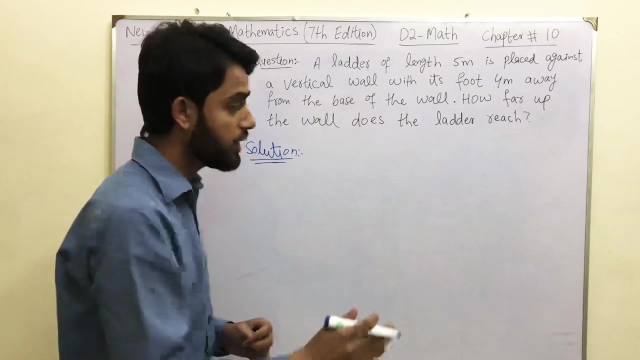 Okay, so I am coming to the solution quickly. You know what actually the idea of solving a world problem like this is: that the moment you are going to solve a problem, You are reading your question and the second you have to draw a figure. let's suppose that you have read the first part of the question and you, somewhere, you feel that you need to draw a figure. 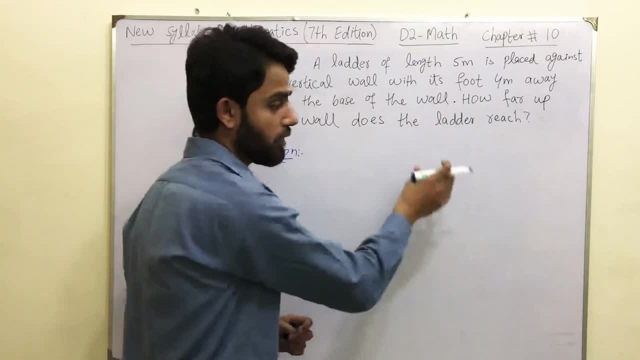 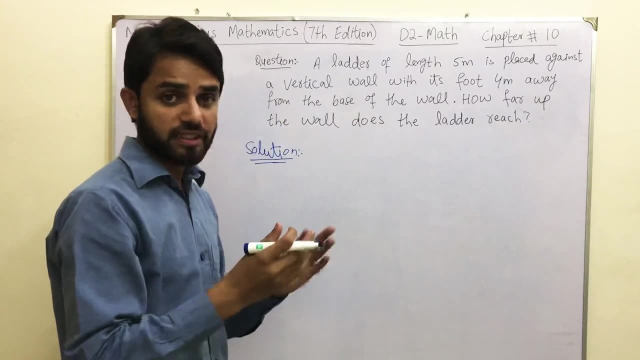 So you have to go step by step. read one part of the question, draw the figure. read second part of the question, complete your figure and see what is being given and what is actually required. So these are the things that I have been continuously emphasizing on all of you: that this is a technique to solve the world problem. 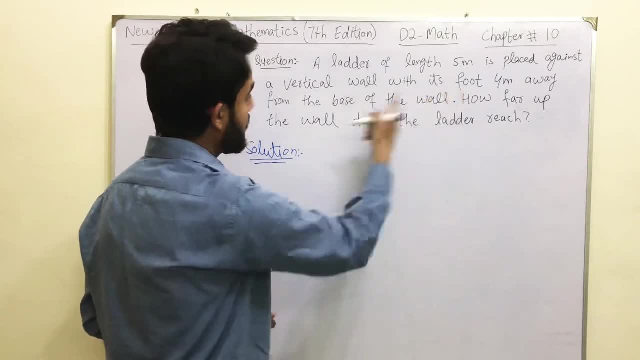 A ladder of length 5 meter is placed against a vertical wall, with its foot 4 meter away from the base of the wall. How far up the wall does the ladder reach? A ladder of length 5 meter is placed against a vertical wall. 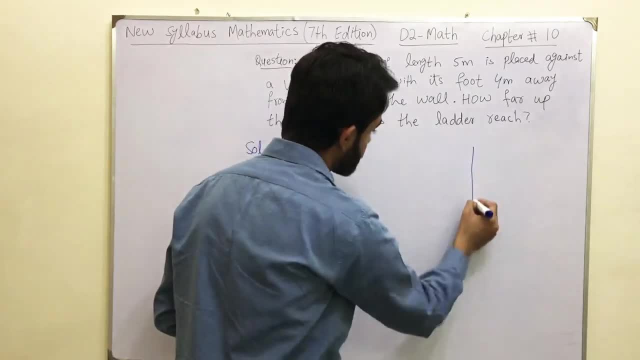 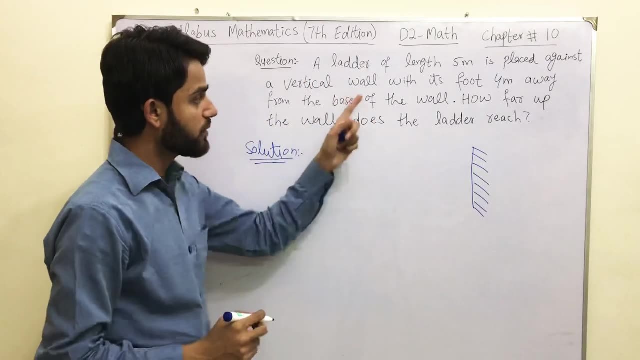 So first of all, we need to make a wall over here. Let's suppose that this is your wall. Now they are saying that a ladder of length 5 meter is placed against a vertical wall. Against a vertical wall means that the ladder is placed like this: 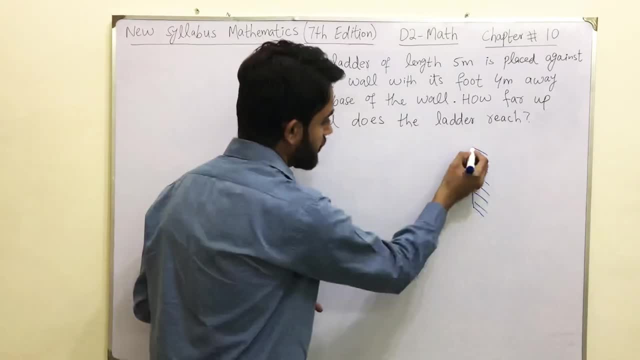 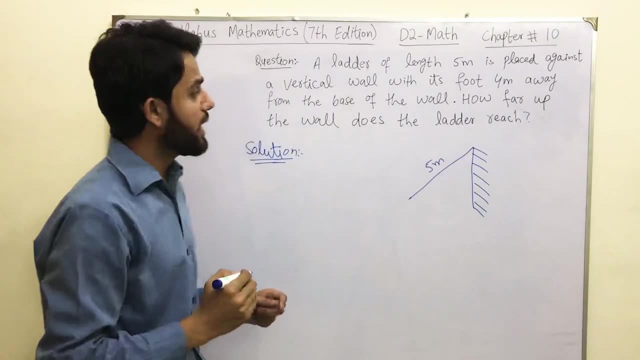 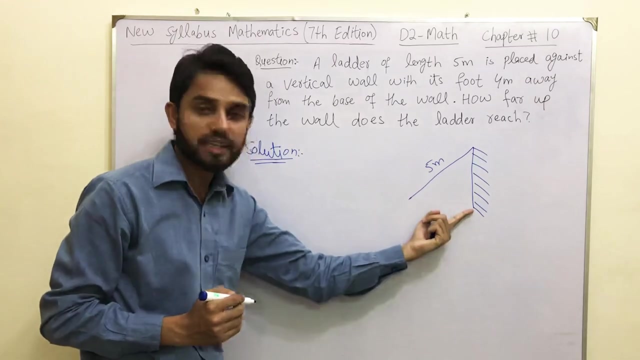 Now, the length of the ladder is 5 meter. How much 5 meter? Okay, this is the length of the ladder And they are saying that with its foot 4 meter away from the base of the wall. So this is basically the base of the wall and this is the foot of the ladder. 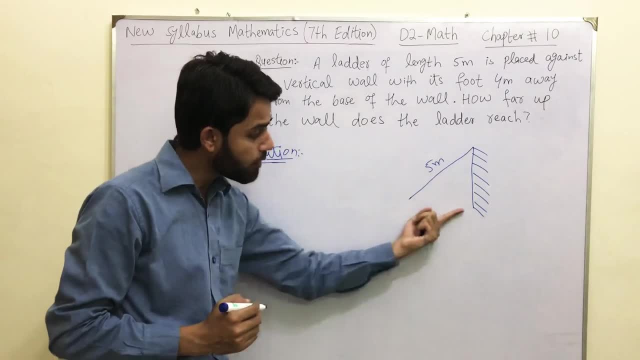 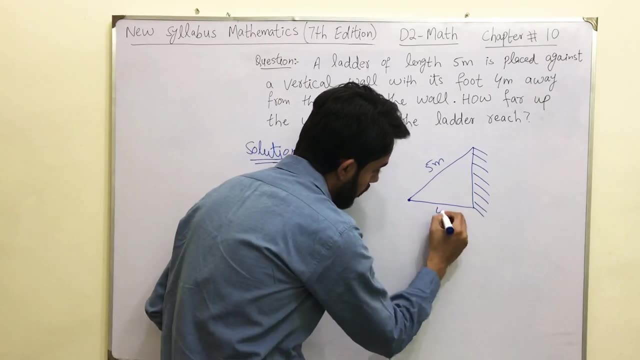 They are saying that this foot of the ladder is 4 meter away from the wall. It means that the distance from this foot of the ladder to the base of the wall is 4 meter. You got it. You see, this is the way that to solve a world problem. 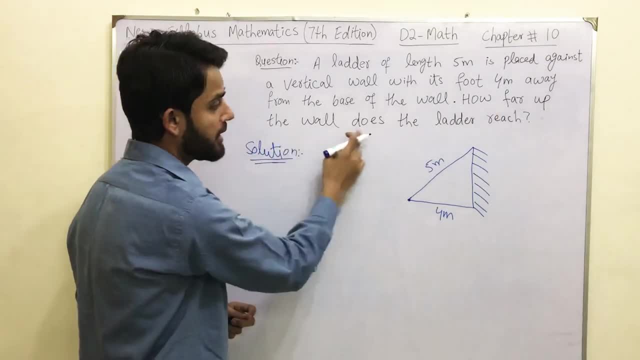 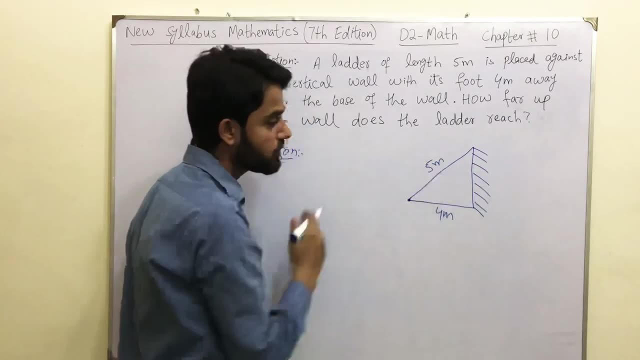 Now third part: How far up the wall does the ladder reach? So it means that you need to find out this height, that how much far this ladder is reaching to the wall. So this is the height that you need to find it out. 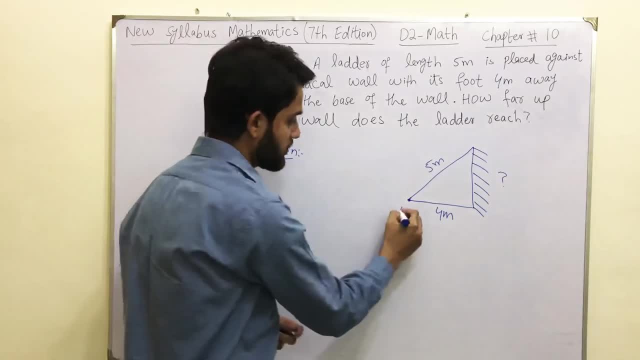 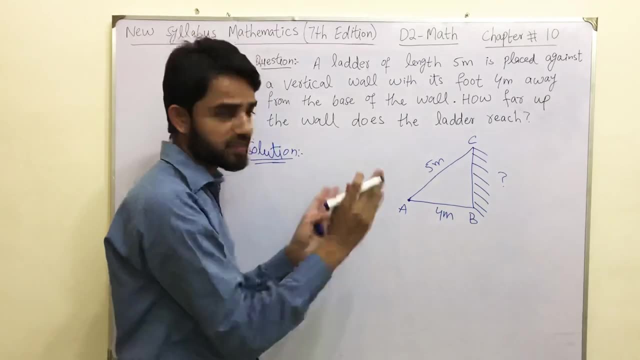 So I am going to give this triangle name. This is your point A, this is your B and this is your C, And if you look at this triangle closely, you will realize that this is a right angle triangle. Why right angle triangle? 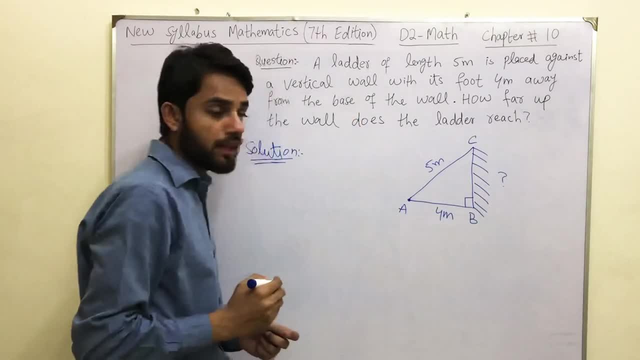 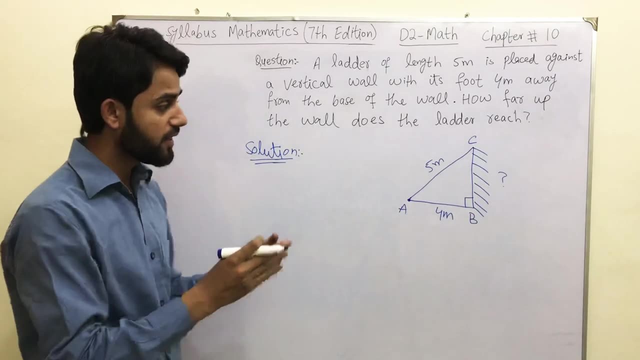 Because over here we have an angle of 90 degree. So now we first need to understand. In order to apply the Pythagoras formula, you need to understand that where is your base, where is your height and where is your hypotenuse. 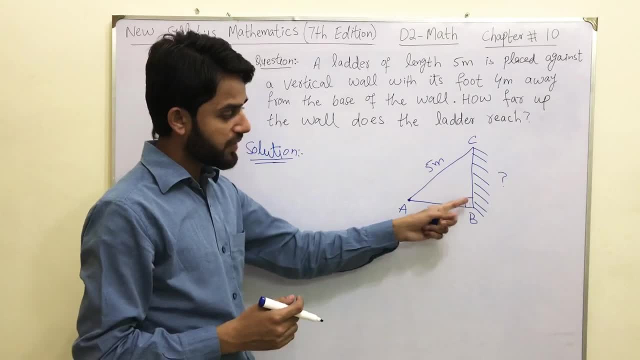 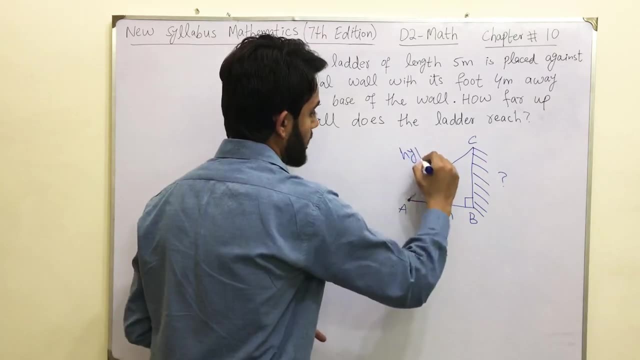 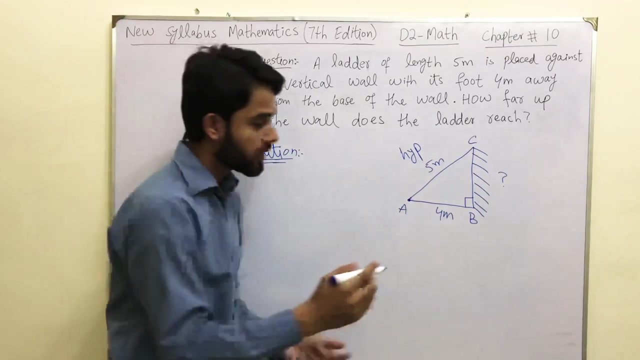 If you got that, where is the angle of 90 degree Opposite to the 90 degree? you will always have hypotenuse. So I am going to write HYP, which will represent height. We just got that and this is the base of the triangle. we can clearly see. 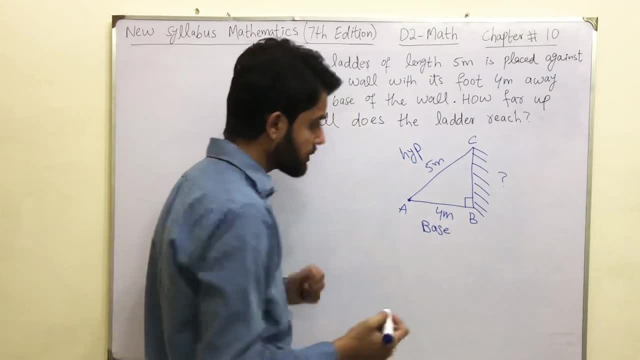 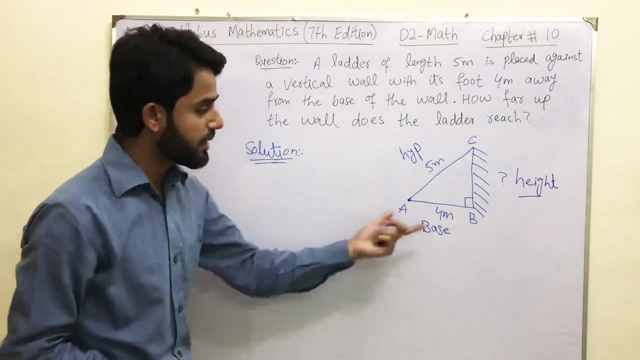 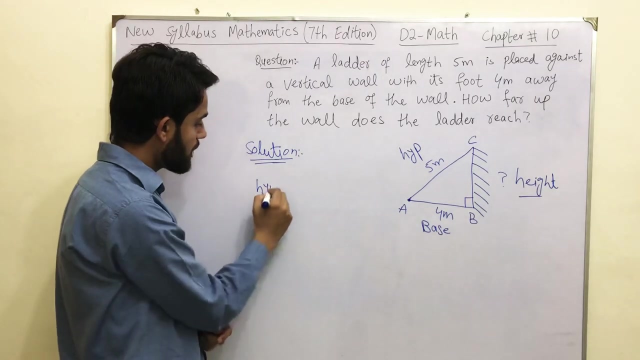 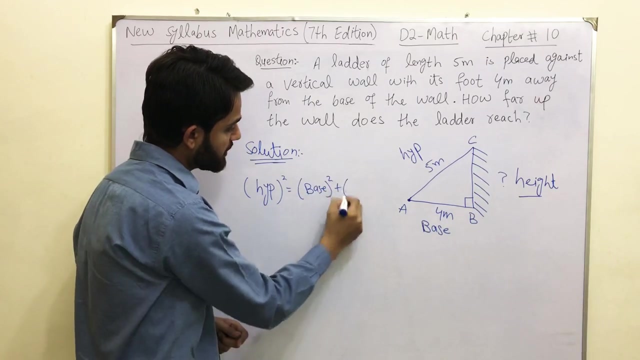 And this is the height. So we just got that in right angle triangle base hypotenuse and this is our height. So we just need to apply the Pythagoras formula, Which is: hypotenuse square is equals to base square plus height. 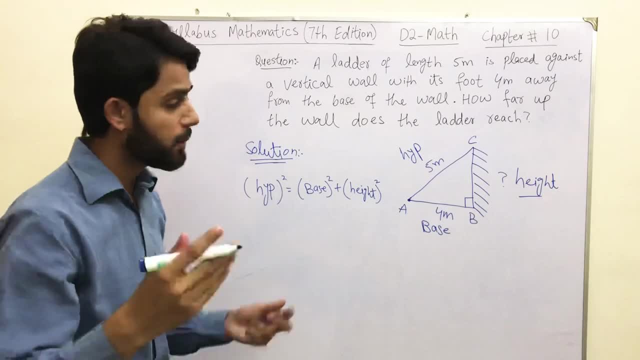 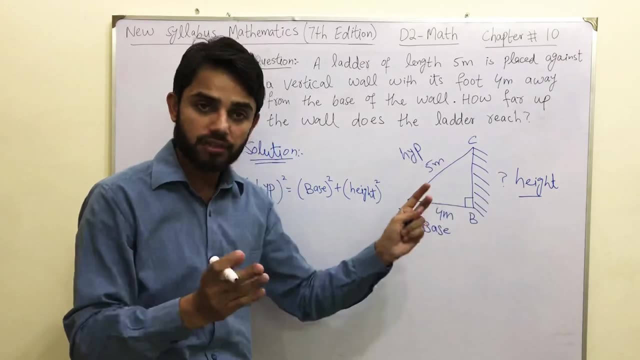 Don't be confused in one thing: Somewhere I will might, or some of the books might, mention this as a perpendicular. So perpendicular and the height, both are the same thing. Alright, If somewhere you have seen that they haven't mentioned height, they are writing perpendicular. 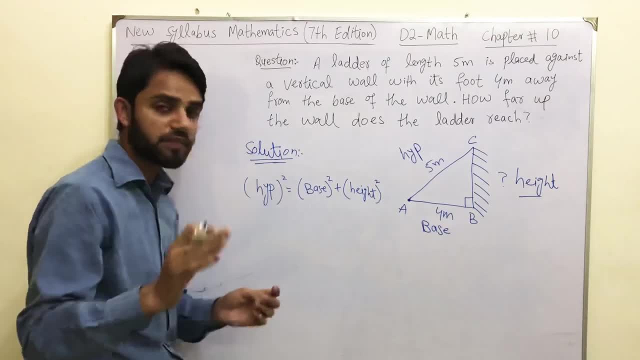 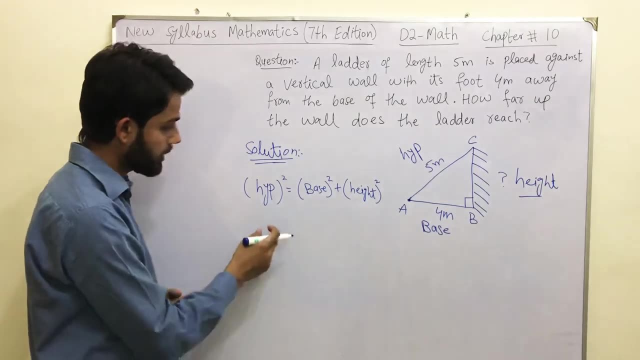 So both are fine, Don't be confused. So if you are still confused, if you have any question, there is a comment box section at the end of the video. You can always comment on it. I will get back to you, So height. 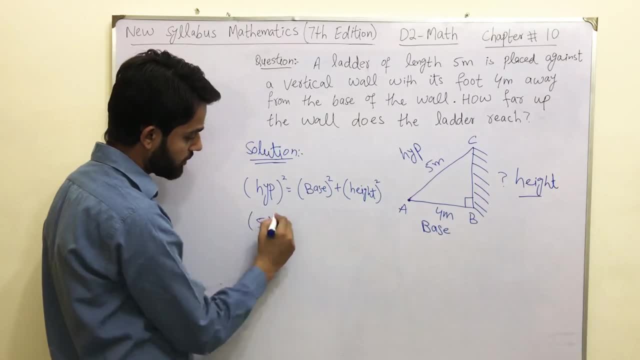 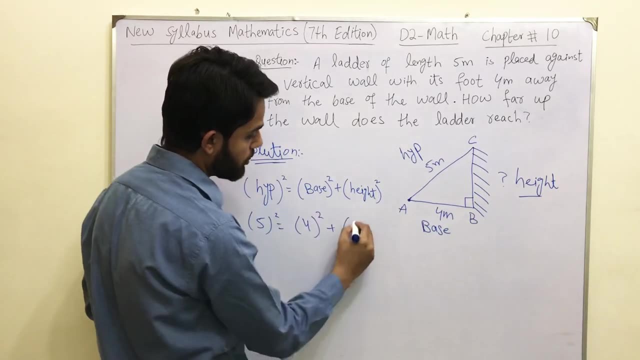 How much height we have? 5. Plug in the value 5 square. How much base do we have? 4. Plus how much height we have. We don't know. This is what we need to find it out. 5 square means that 25.. 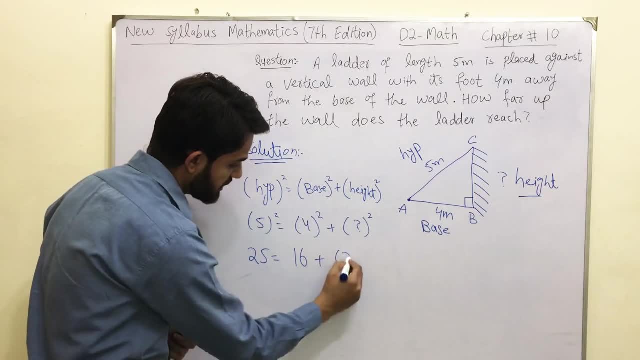 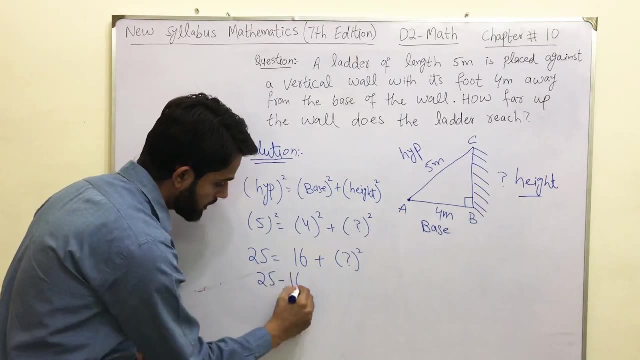 4 square means that 16.. Plus, this is what we have to find it out. Okay, Shift this 16 from here to here. 25 minus 16 is equals to question mark. You can give this name or you can use as a height. 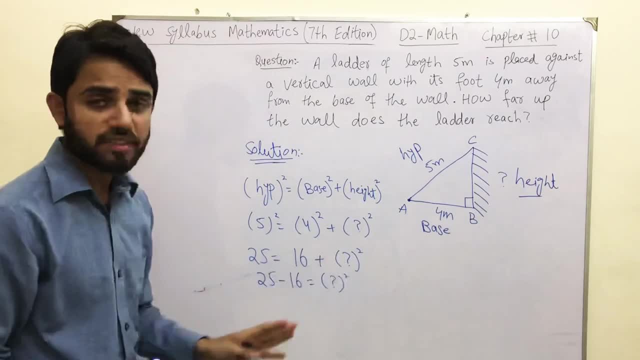 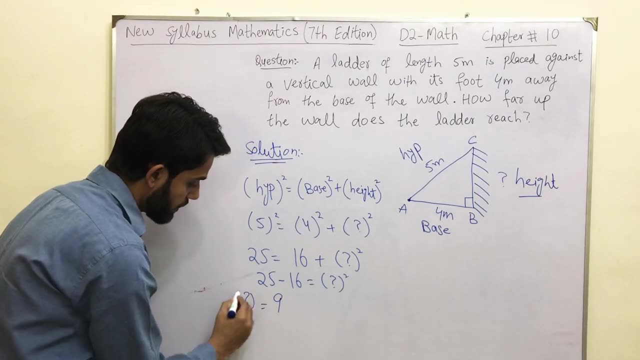 There are infinite many ways where you can represent this Alright. So 25 minus 16 is going to give you 9 is equals to this question mark square. So we need to find out the height. We don't need to find out the height square. 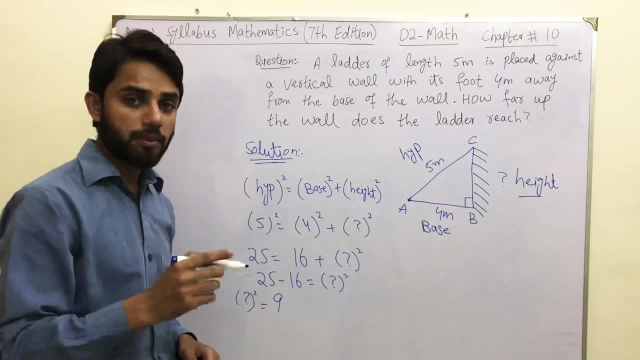 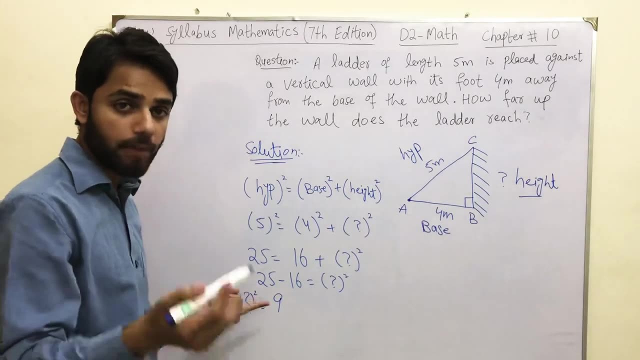 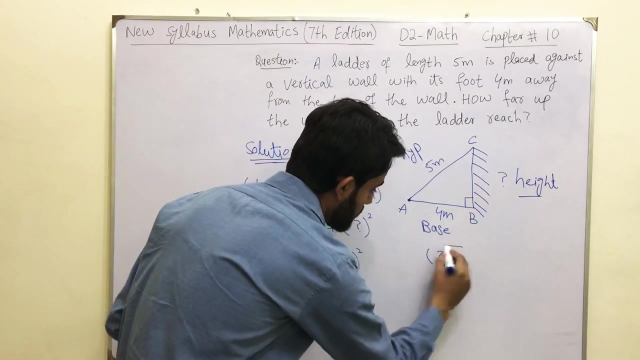 So if you have watched my previous video, then you do remember that we have learnt how to cancel the square from any power or from anywhere. So we got to take the square root on both side of this equation. Over here you have question mark. 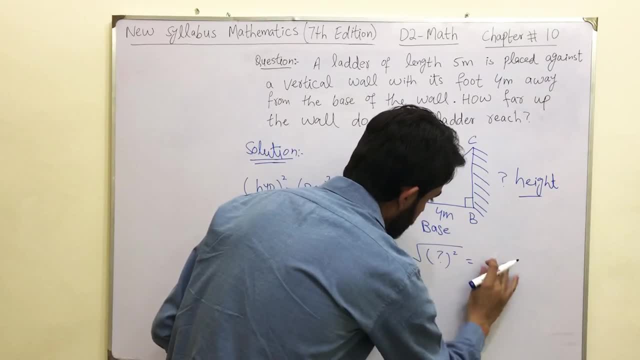 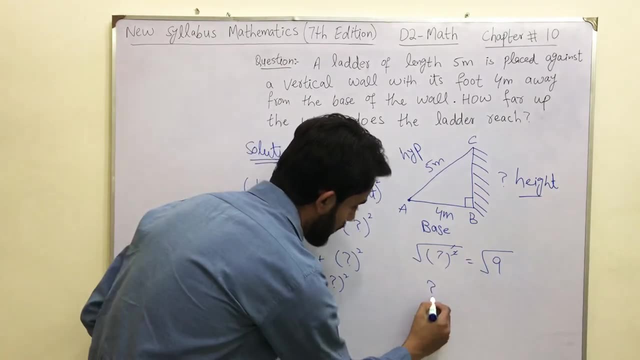 Take this square root. Over here you have 9.. Take this square root. So once you cancel this one, because they both are opposite to each other, over here You are left with question mark And over here square root of 9.. 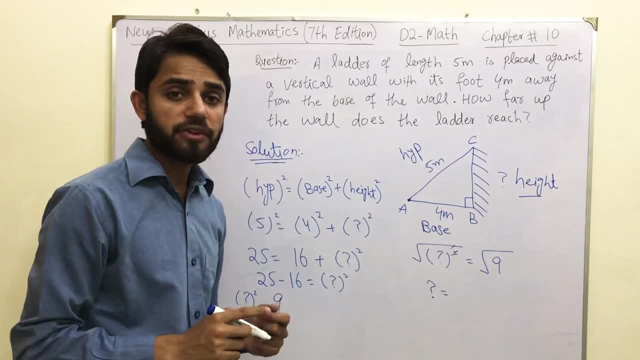 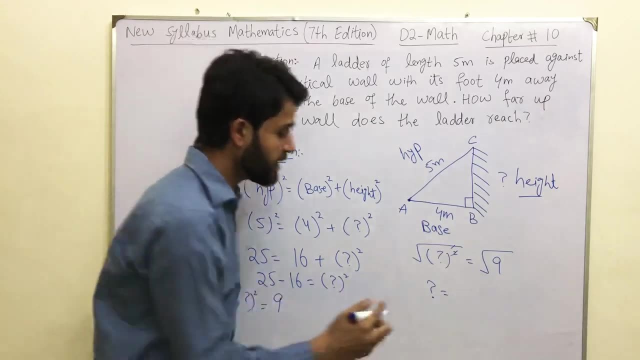 Now I have given you the concept earlier in my video that every time when you remove the square root, You are going to get the two values, Which is positive and negative, Over here. So you will write plus minus 3.. But the thing is that we are finding the height. 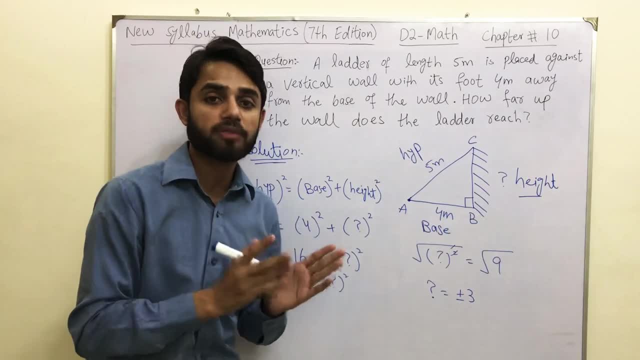 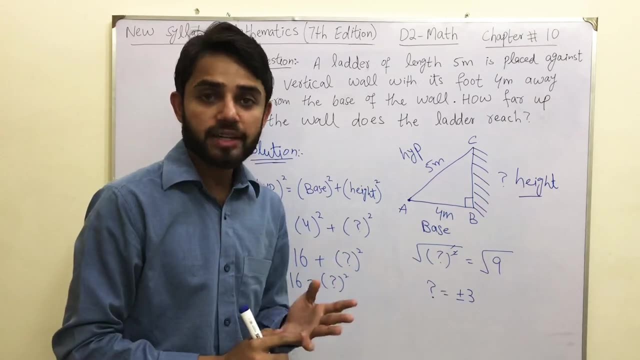 I have also. I do remember that I have also given you the concept on that video. If somewhere you are finding the radius, the diameter, the length of any object, We know that the radius, the diameter, the length can never be negative. 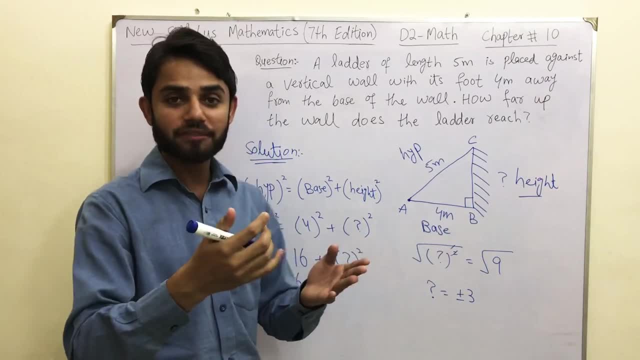 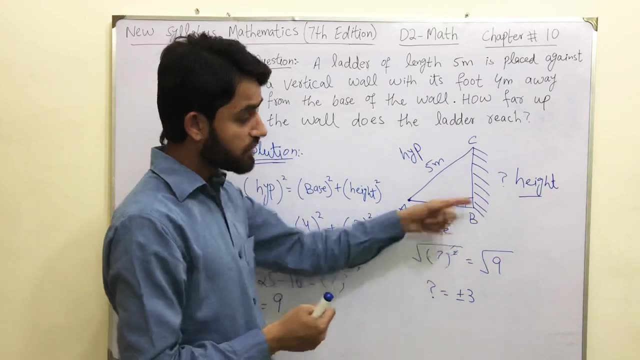 Have you ever heard from someone that someone is walking minus 15 meter? I mean, it's not possible that the distance is going to be negative Or the length is going to be negative. So over here, this is the obvious situation. Yes, positive 3 square is also 9.. 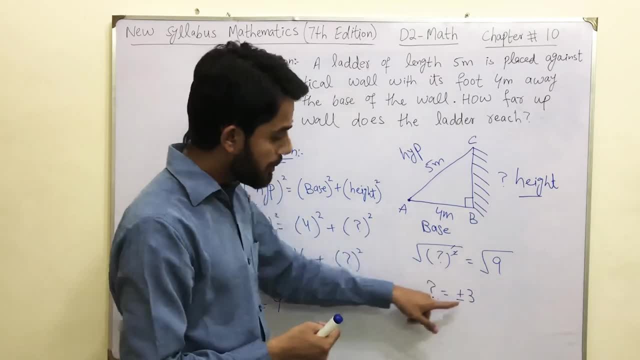 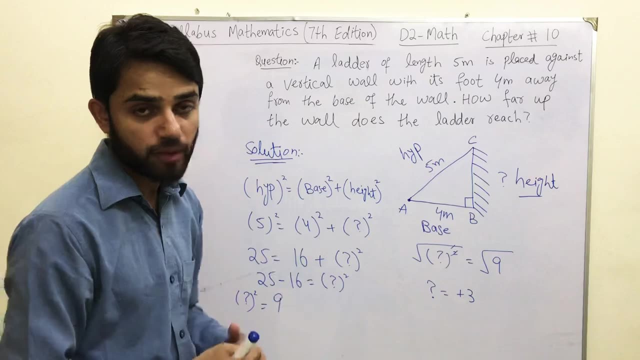 Minus 3 square is also going to be 9.. But over here you can't write minus. Just ignore it, Because you are finding the length and it's never going to be negative. So we have just completed our first step. 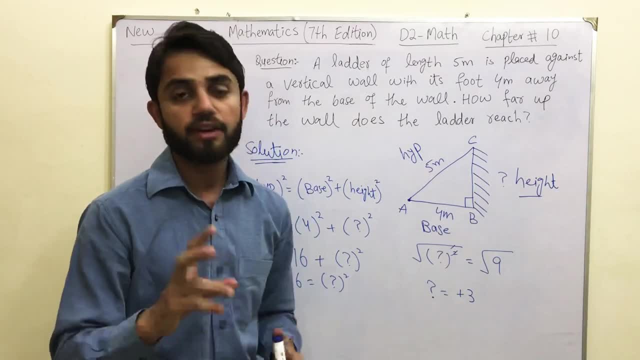 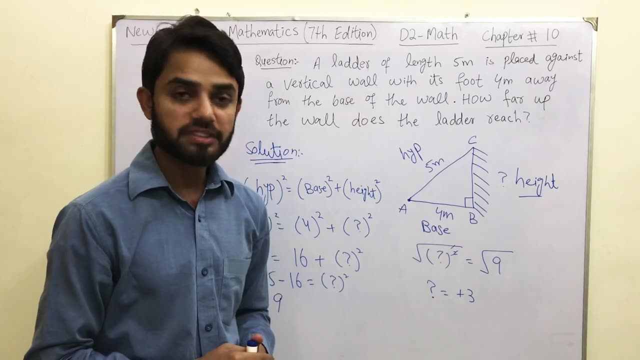 So if you have still confusion, You can get back to me. My business email id is already mentioned on my YouTube channel, So please subscribe this channel and share the videos as much as you can So that I can make much more to help you all.